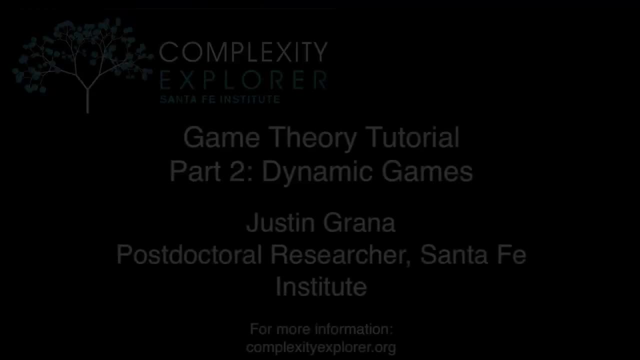 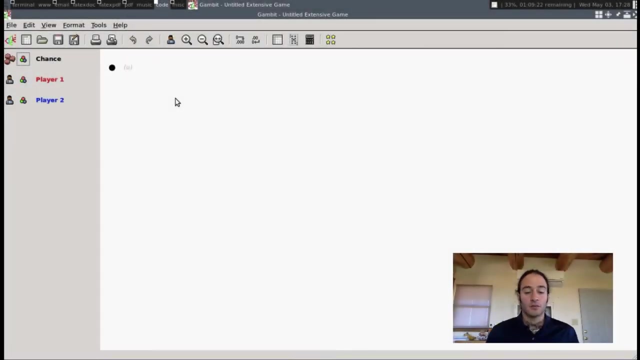 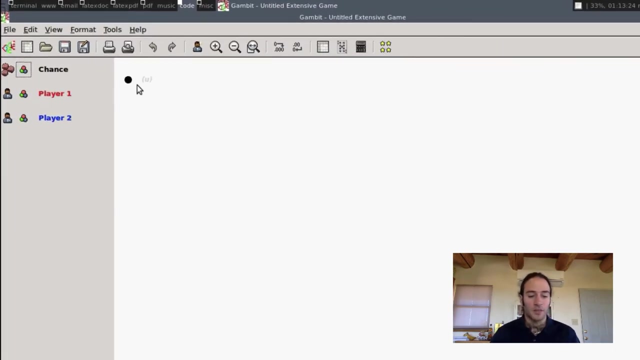 In this lesson and the final lesson of the tutorial, we're going to use Gambit to solve a sequential or an extensive form game. So when you open Gambit you can go to File New and Extensive Game and it will give you this screen. So let's do a simple game. 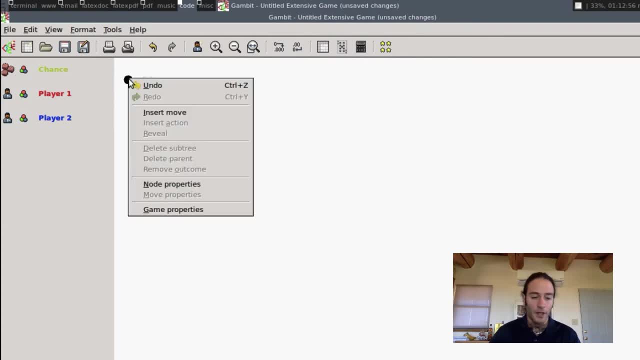 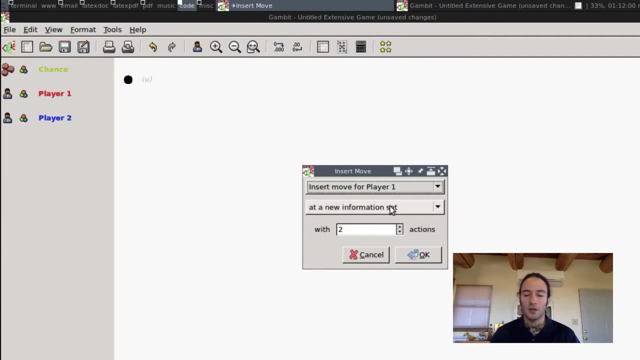 while first Player 1 moves and then Player 2 moves. I'm going to right-click this first node here and insert a move. We're going to insert the move for Player 1.. We're going to do it at a new information set. I haven't touched too much on what information sets. 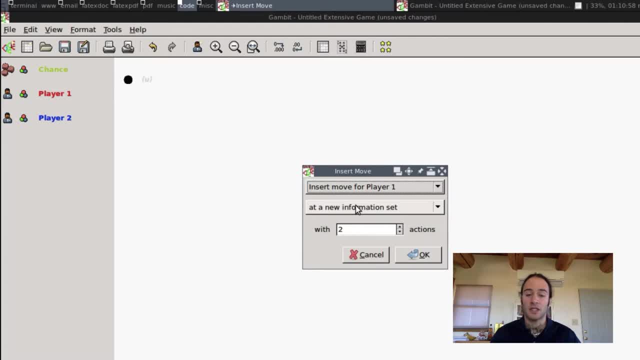 mean, but this allows for imperfect information and players not to know where they are in the game tree. We touched a little bit about this, on this in the first section of videos in Part 1 of the tutorial in Bayesian games. But for now, because everything is going to, 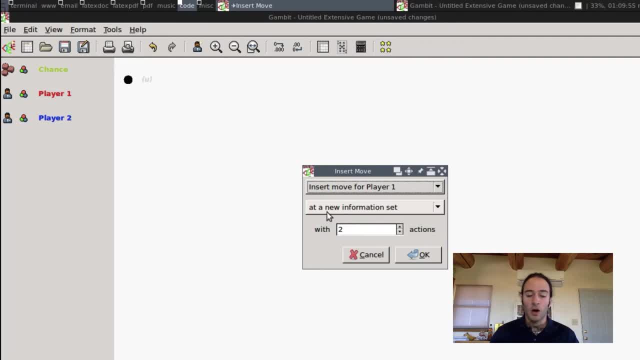 be complete information and players will observe everything that happened before them. we're always going to use Gambit to solve a sequential or an extensive form game. We're going to do it at a new information set and we're going to let Player 1 have two actions. Let's 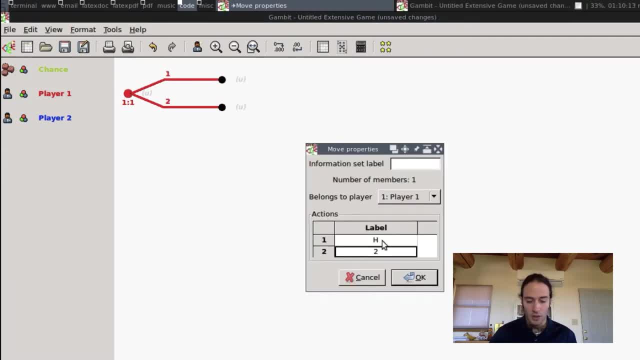 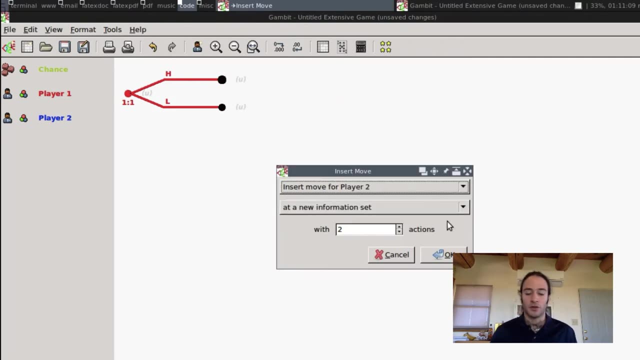 label his actions just simply: High, H and L for Low. Now, after Player 1 acts, after choosing H or L, we want to let Player 2 do something, So we go to Insert Move for Player 2.. Again, we're always going to do it at new information sets and we're going to give 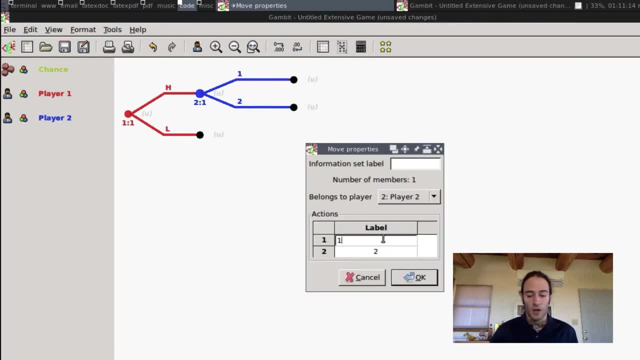 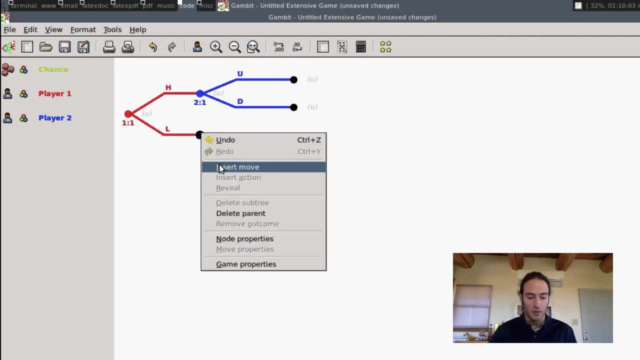 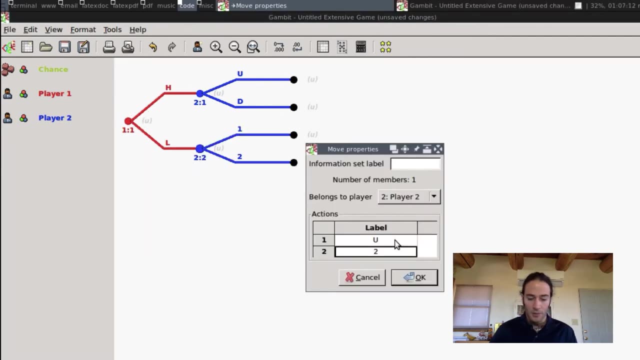 him two actions And similarly, we'll call, I guess, his action Up, And we're going to do the same thing here And we'll call his actions again Up and Down. Now the last thing to put in are payoffs, And I'm just going to enter some numbers. You just double. 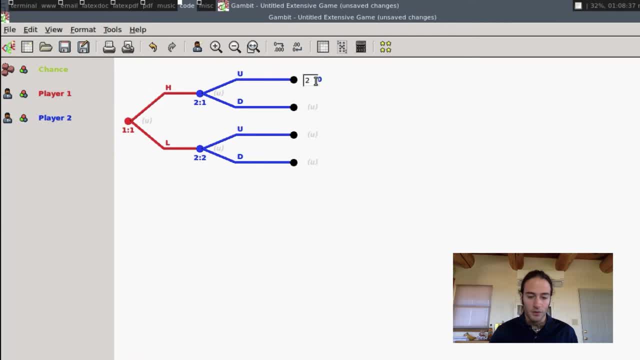 click here where you see the little U And I don't know, first number 2,, second number 1.. And this means that if Player 1 plays H and Player 2 plays U, then Player 2 plays U. Player 1 gets a payoff of 2.. Player 2 gets a payoff of 1.. It's nice here that everything. 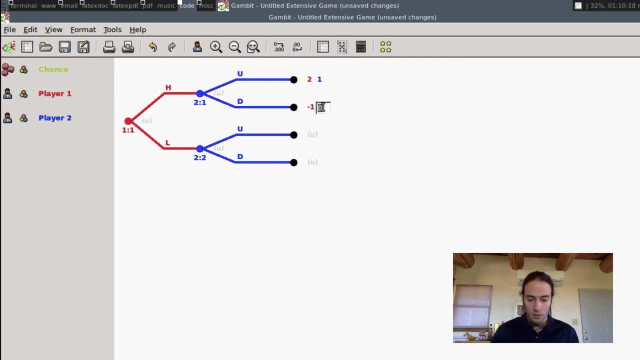 is color-coded for you. I'm just entering some random payoffs so we can see how this works. Oops, Okay, So now we just go to Tools- Equilibrium. and then we're going to go to Equilibrium. We're just going to compute 1 once again, Hey, And we get an equilibrium. 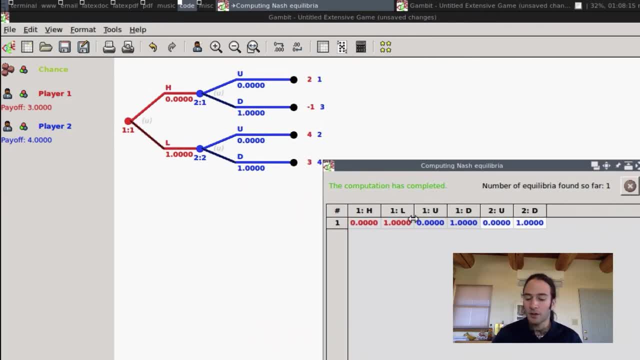 So what does this say? So remember, red is Player 1, blue is Player 2.. So this says: Player 1 at information set 1, that's what this 1 means. he should play L with probability 1 and play heads, or sorry. L which means low with probability 1, and H, which means high. 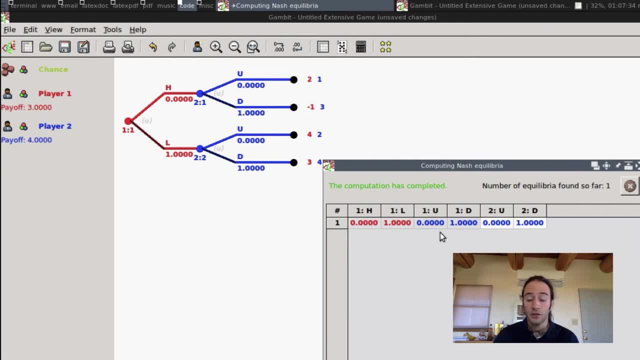 with probability 0.. Now, remember, Player 2 has to condition on what Player 1 did. So what this says is: if Player 1,, I'm sorry, if Player 2- is at its first information set, which is this up here: 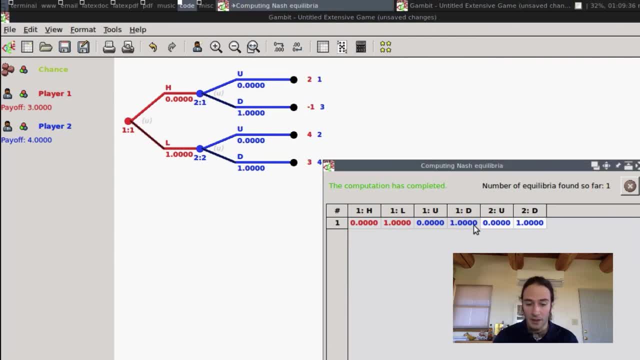 when Player 1 played H, Player 2 should play D. And this makes sense, right? Because if Player 2 finds itself here, then it should play D, because it prefers 3 over 1.. Similarly, this here says Player 2.. 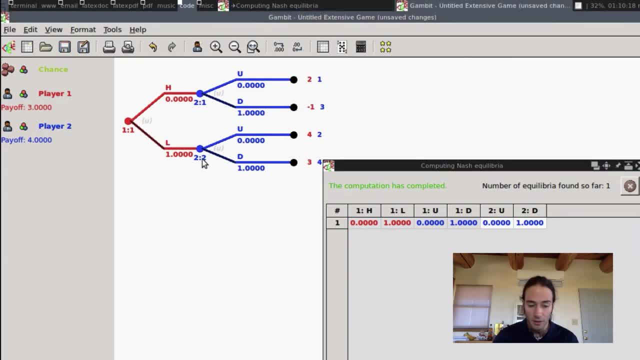 Player 2 at its second information set. note here 2, its second information set, which corresponds to player 1 playing low, should play up with probability 0 and down with probability 1.. And what this means, once again, is that okay if player 2 finds itself here? 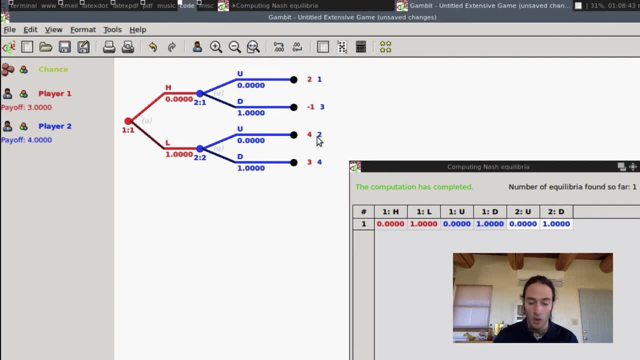 it should play down because it prefers 4 over 2.. So in this case, Gamut has solved for a Nash equilibrium. in this game, As an exercise, we're going to see if Gamut solves for sub-game perfect equilibria. 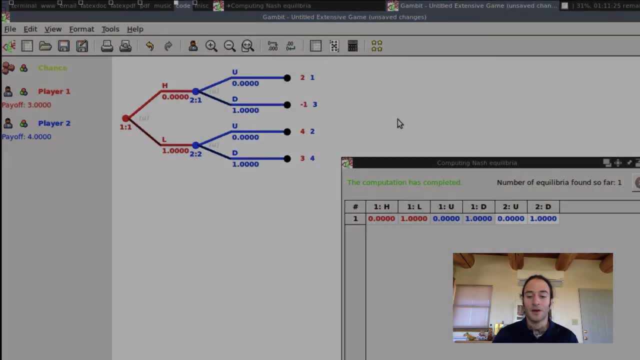 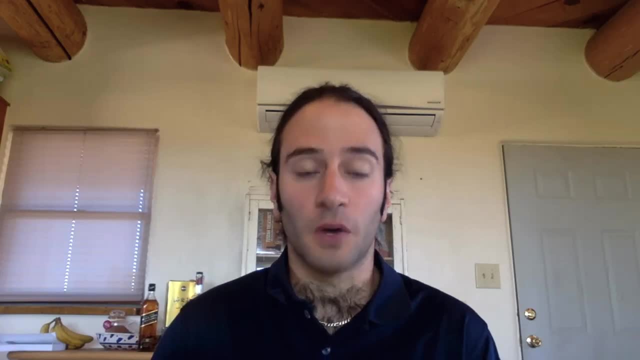 especially when you let it solve for all equilibria. I hope you enjoyed that one. Thank you everybody for sticking with me on this second tutorial of game theory. I hope you enjoyed both the first set of videos and second set of videos. 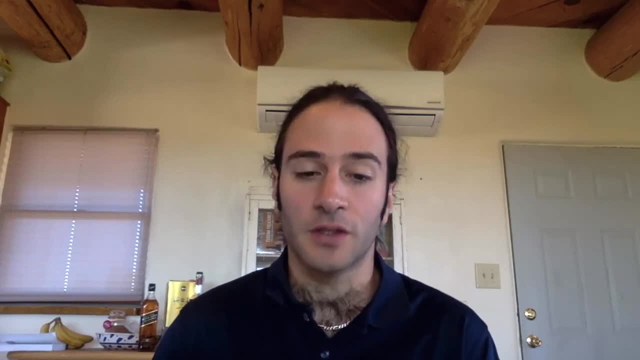 And I hope that you learned something that you can apply to your daily life as well as your studies in complexity. Thank you very much.